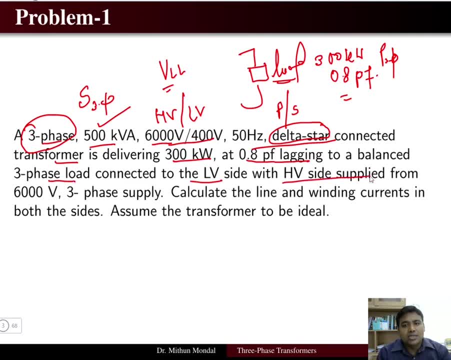 three phase load connected to the low voltage side with high voltage side supplied from 6000 volt. So high voltage is supplied from 6,000 volt and 400 volt. the load is connected. Now calculate the line and winding currents in both the sides. So you have to calculate. 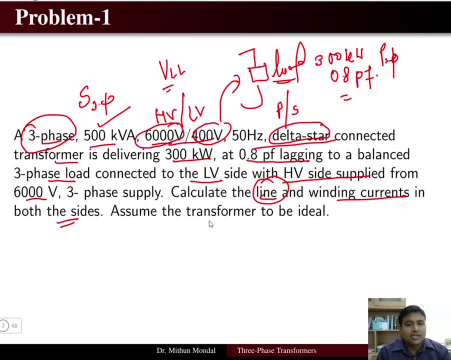 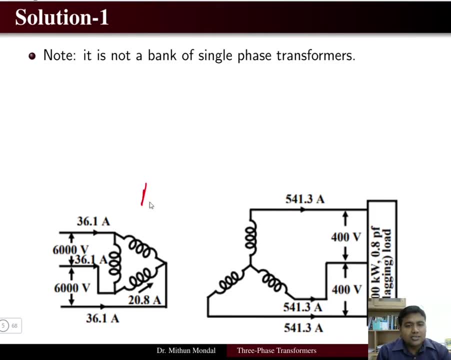 what is the line current and what is the phase current when both the sides Assume the transformer to be ideal. so let us see the solution. so here we have a delta- star connected transformer. so we have been given a delta connection transformer and star connected transformer. so delta is on the 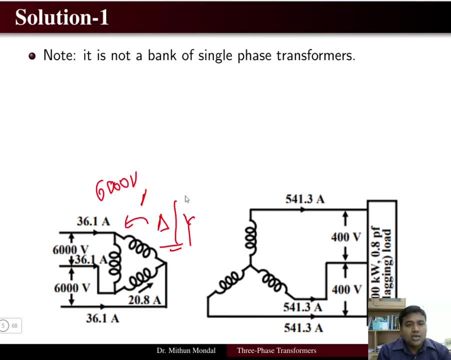 high voltage side, which is around 6000 volt, and star connected side is 400 volt transformer. now you have to make a special note that it is not a bank of single phase transformer, but it is a three-phase transformer as a single unit. so here you have a three-phase transformer. 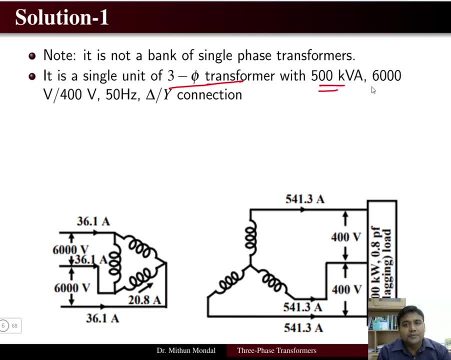 as a single unit with the rating 500 kva, 6000 by 400 volt, 50 hertz delta star connected transformer. so it means that 500 kva, whatever the rating is given, is the total kva of the three-phase system and the voltage that is being given, 6000 by 400 volt. it is corresponding to line to line voltage. 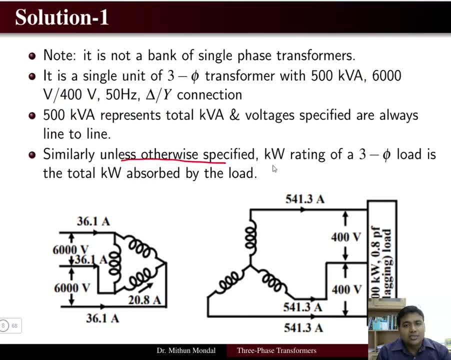 and similarly you have to make a three-phase transformer as a single unit. so here you have a three-phase transformer as a single unit but, unless otherwise specified, the kilowatt rating of the three-phase load. so the load that is being information is given to you- is basically the three-phase. so 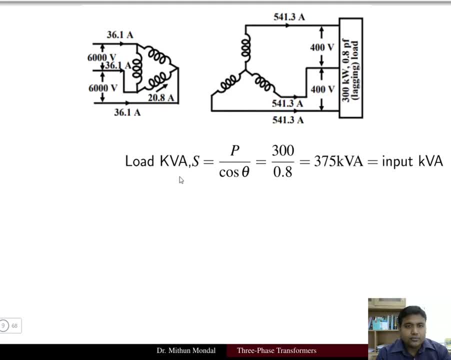 total kilowatt absorbed by the load is given. now, in order to find the current, and in the three-phase and the phase current, we will use the kva. so we know that the load kva formula s is equal to p by cos theta, where p is the real power, s is the apparent power and cos theta is the power. 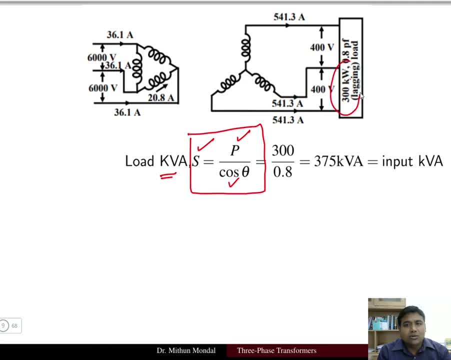 factor. so here we have been, given that the real power is 300 kilowatt divided by 0.8, that is, the power factor, is 375 kva. so the output, that is the 375 kva. so the input of the transformer has to be. 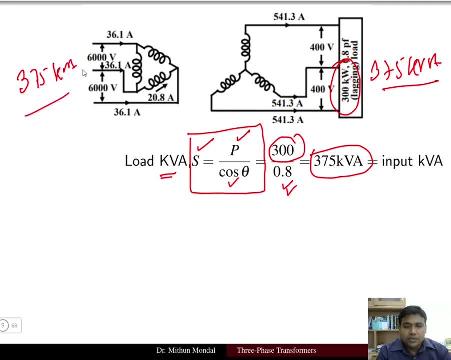 also 375 kva. okay now, so we can find what is the current flowing in the line current of the secondary. so line current drawn by the load, we can find the current flowing in the line current of the secondary from the formula that the complex power s is equal to root three times the vl line voltage. 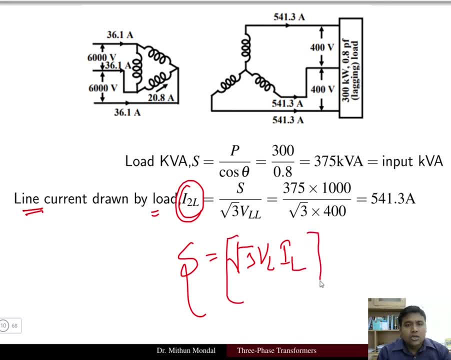 into the line current. so we have been given the complex power as 375 kva, which we have estimated, and the line voltage is given to us is 400 volt. so on substituting the values of the complex power and the line voltage, we can get the line current. 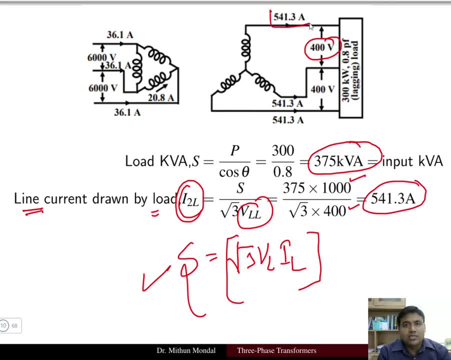 as 541.3 ampere. so 541.3 ampere is the current which is flowing to the load and this is three phase. now on the high voltage side. if we take this on the high voltage side, then we can calculate that from the high voltage concept. so we have a 6000 volt voltage and the power is 375 kva, which is the. 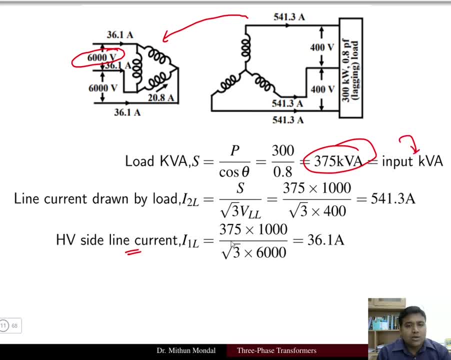 input power. so we can substitute the complex power 375 into 1000 divided by root, 3 into 6000 volt as the input voltage and this is the line voltage. so whatever the current, we are obtaining 36.1 ampere. that is basically the line current on the high voltage side. so 36.1 ampere. 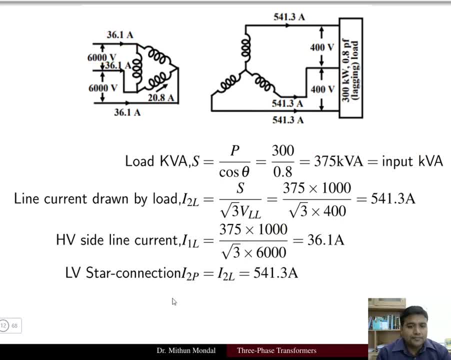 will be the current which is flowing on the high voltage side of the transformer. now this is basically delta connected and this is star connected and we can apply the concept of the voltage for the star and the delta. so we know that the phase current is equal to line current. in case of the star connected machine, which is the low voltage side of 400 kva. so on the 400 volt side the current will be 541.3 ampere because it is star connected system. so we know that line current is equal to phase current for a star connected system. so here the phase current will be 541.3. 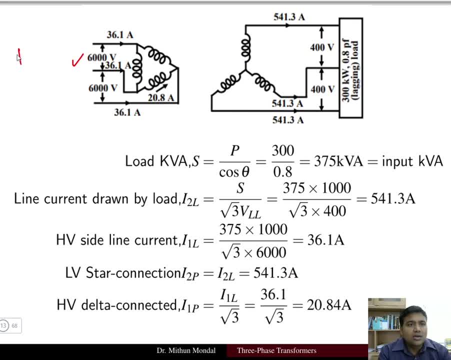 whereas on the high voltage side here we know that the line current is equal to root 3 times the phase current for a delta connected machine. so phase current we can calculate as line current by root 3, and we have already obtained 36.1 ampere as the line current. so 36.1 ampere divided by root 3. 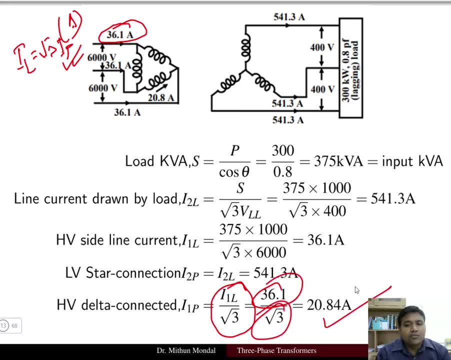 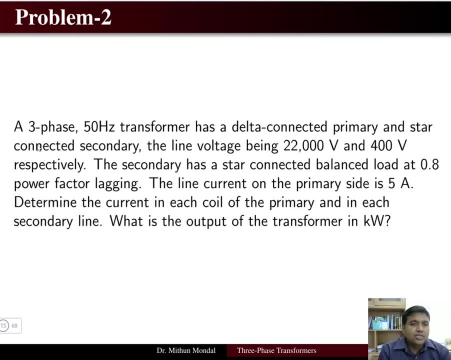 will give you 20- 20.84. so 20.84 is the phase current which is flowing on the high voltage side of the transformer. next problem that we are going to deal is a three phase 50 hertz transformer has a delta connected primary. so primary side is delta. connected and star side is secondary, secondary side is star connected. so basically the transformer can be written as delta star connected transformer, the line voltage being 22, 400 volt respectively. so here you have: the primary is connected to 22 000 volt and secondary is connected to 400 volt. the 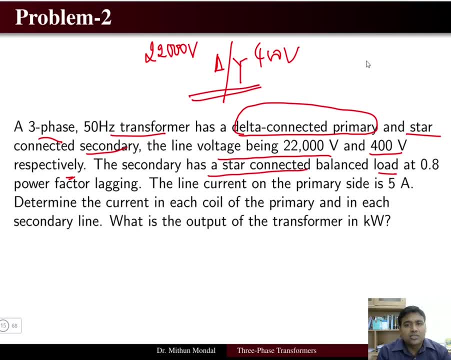 secondary has a star connected balanced load. so the load information is given, which is a star connected load and it is at 22.8 power factor lagging condition. so this is the information of the load. the line current on the primary side is 5 ampere. so basically the current that is flowing on the primary and the 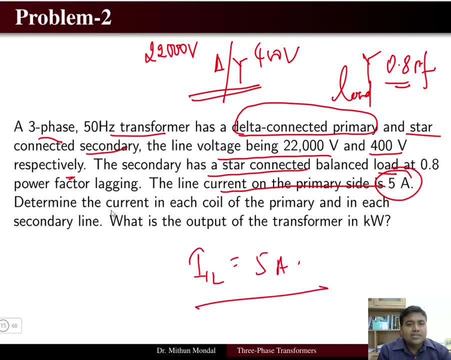 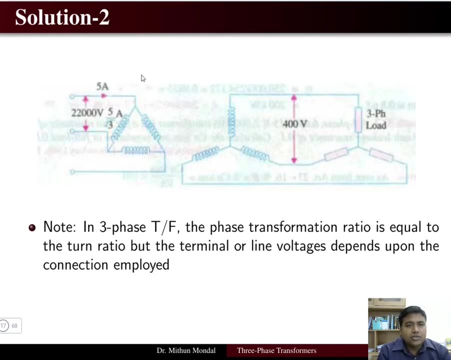 line current is 5 ampere. determine the current in each coil of the primary and each secondary line. what is the output of the transformer in kilowatt? so power output we have to calculate and the current we have to calculate for the coil. so let us see and draw the diagram. so first, 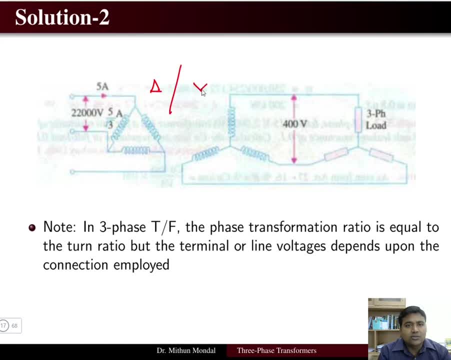 on the primary side we have Delta connected and on the secondary side we have star connected. the Delta connected is giving a line voltage of 22 000, whereas the star connected we have a voltage of 400 volt and there is a three-phase load which is basically star connected, so in three phase. transformer. the phase transformation ratio is equal to the turns ratio, but the terminal or line voltage depends upon the connected equal. so depending upon what type of connections you give- and Delta or a star- the correspondingly voltage and current will be dependent. but the transformation ratio we have to obtain based on the turns ratio. so phase voltage on the primary. 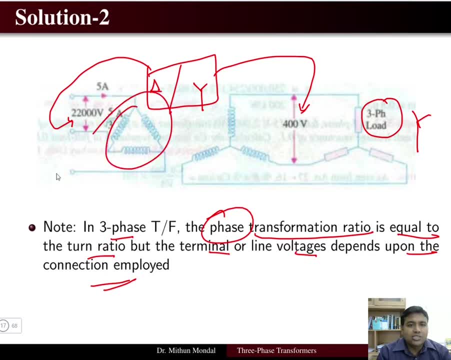 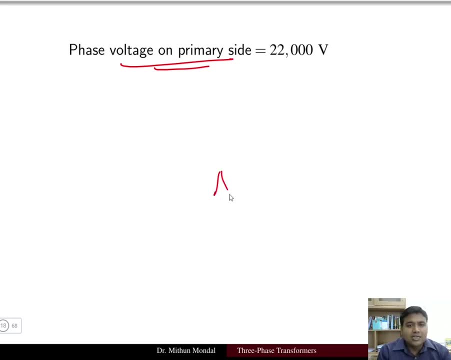 side. so our primary side is basically Delta connected machine, and twenty two thousand is the line voltage. so the we know that in Delta connected machine we know that line voltage will be equal to phase voltage. so line voltage is twenty two thousand, so phase voltage become equal to 22,000 on the primary side, Whereas on the secondary side, since it is a 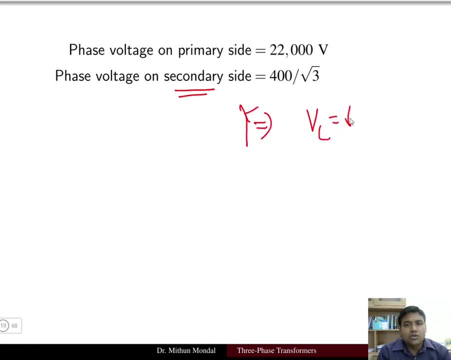 star-connected machine. we know that line voltage is equal to root 3 times the phase voltage. So we can obtain: the phase voltage is equal to line voltage by root 3.. So 400 volt, whatever is flowing on the secondary side, you divide it with root 3, you will get the phase voltage. 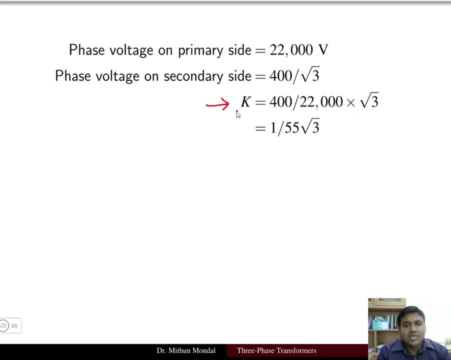 Then the transformation ratio. we can obtain k, depending on the phase voltage of the primary side and the secondary side. So on the secondary side we have 400 by root 3 and on the primary side we have 22,000.. So this will give you the transformation ratio or the phase transformation. 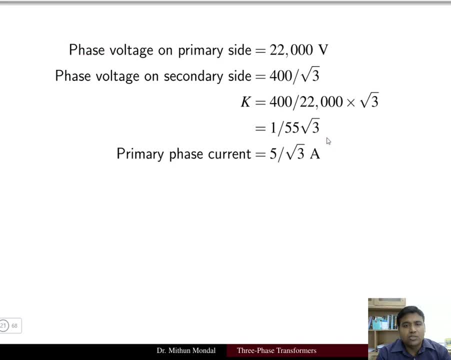 ratio. So you will get 1 by 55 root 3.. Then the primary phase current. so on the primary side your connection is basically delta-connected machine and we know that line current is equal to root 3 times the phase current. So phase current we can obtain as: 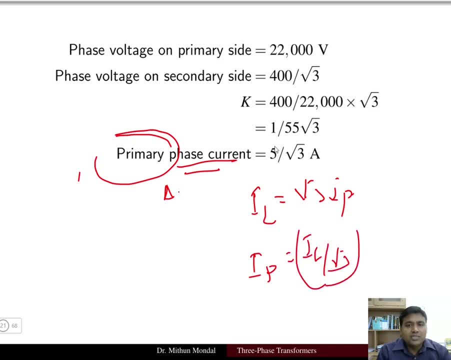 line current by root 3.. So we have been given 5 ampere is the current which is flowing in the line. So divided by root 3 will give you the phase current on the primary side. Secondary side we can obtain from the relationship: k is equal to the current that is flowing I1 by I2.. 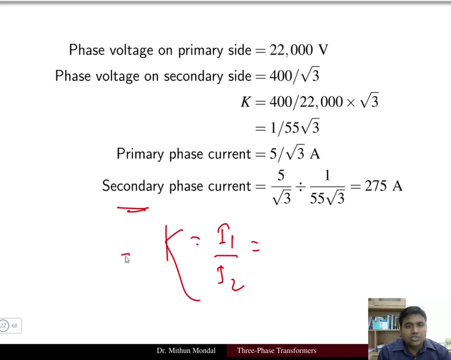 I2 is equal to the transformation ratio. So, transformation ratio, you have obtained this much, and we have also obtained the value of the primary current, I1, as this much. So, substituting the value of I1 and k, we can get what is the value of I2.. So I2 phase current will come to be 275 ampere. 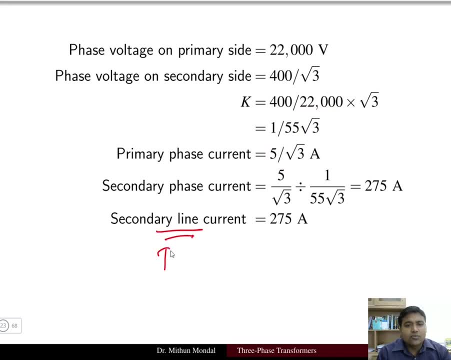 Then the secondary line current. so what is the current that is flowing in the secondary line? So, since it is a star-connected machine, in star-connected machine we know the line current and phase current are one and the same. So line current and phase current will be same in star-connected machine. So 275 ampere. 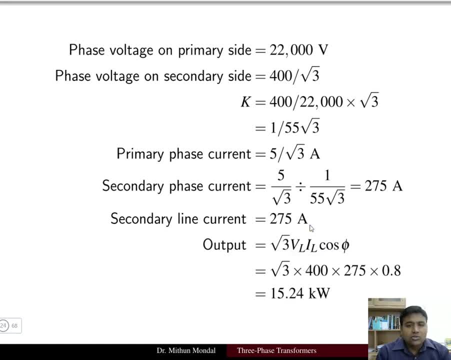 will be equal in both the cases. Now the output power that we have to calculate. so the power has to be calculated in kilowatt, So the formula will be: root: 3 VLi cos phi or otherwise. we can also put 3 phi, phase I, phase, cos phi, Anything we can put. So in terms of the 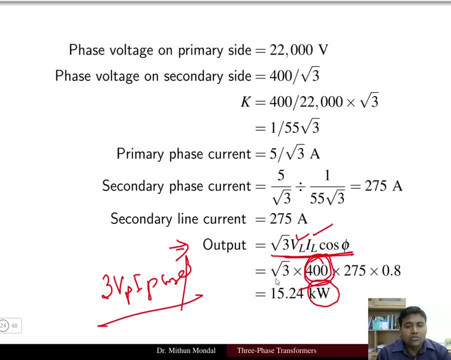 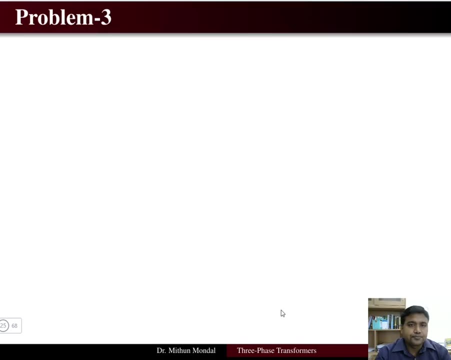 line voltage, if you want to calculate, because 400 volt is the line voltage on the secondary side and 275 ampere is the current which is flowing on the line side. this one and the power factor is 0.8.. So that gives you 15.24 kilowatt as the output power. Next problem: we have a 500 kVA. 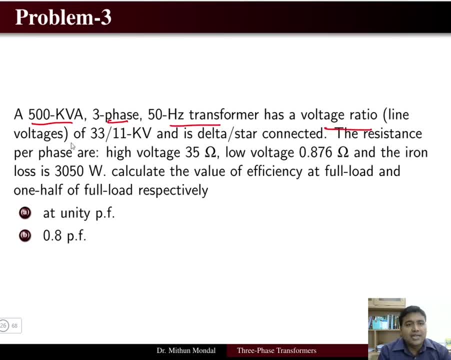 3 phase 50 hertz transformer. voltage ratio: line voltages of 33 by 11 kV. So that is a delta connected machine. So on the primary side we have delta connected, On the secondary side we have star connected. So this is around 33 kV and this is 11 kV. Power rating is 500 kVA. 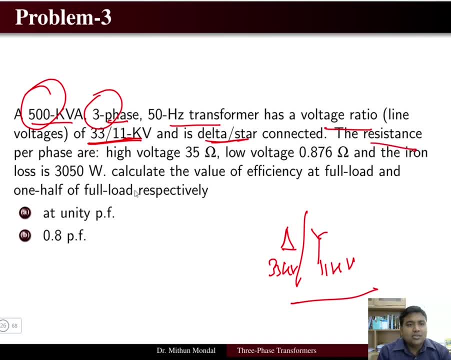 corresponding to 3 phase. Now the resistance per phase. So always the parameters will be given per phase basis. All the parameters will be given per phase basis. So the resistance on the high voltage side, So high voltage side is 33 kV side, So it is 35 ohms. 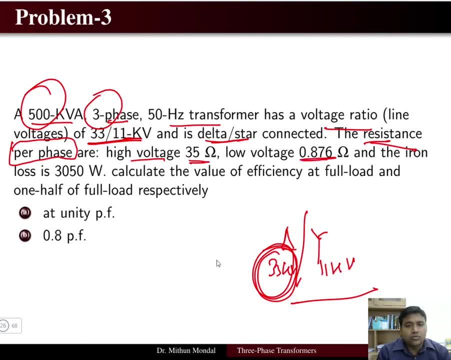 And on the low voltage side is 0.876 ohms. So here you have 35 ohms and in this side you have 0.876 ohms, Iron loss being given as 3050 watt, So you have an iron loss of 3050 watt Calculate. 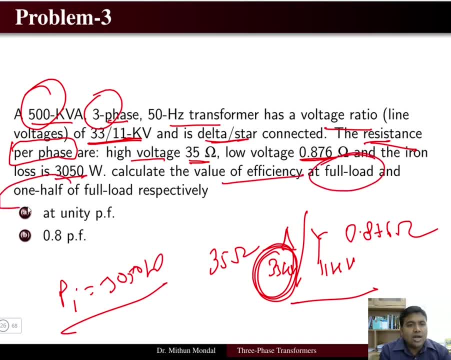 the value of efficiency under the full load condition and one half of the full load condition at different power factor. One is unity power factor and 0.8 power factor. So iron loss is constant loss, It will not depend upon the loading, whereas the copper loss we have to calculate. 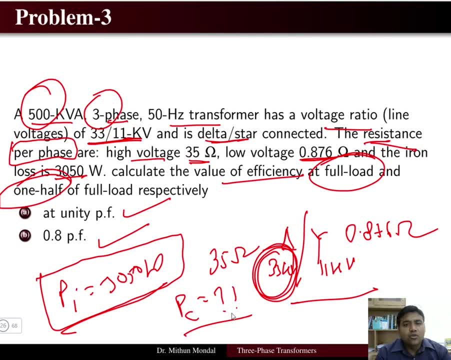 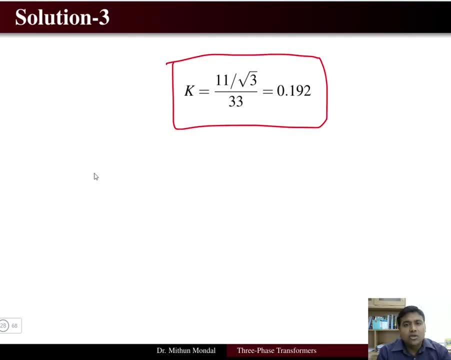 and then we have to find out at different loading what is the copper loss. So it starts from the transformation ratio. So transformation ratio on the secondary side, we have 11 kV, which is the star side, and this you convert it into phase voltage. So phase voltage on the secondary side. 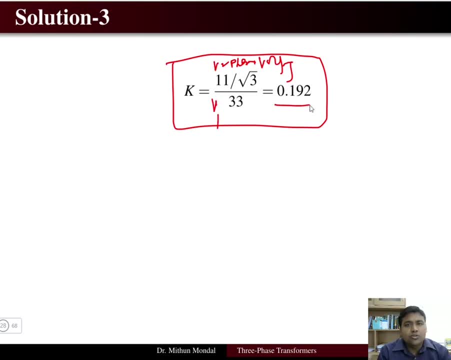 so V2 by V1 of the phase voltage will give you 0.192 as the transformation ratio. Then we will transfer all the parameters on the secondary side, R02.. So R02 will keep the R2 as constant and we 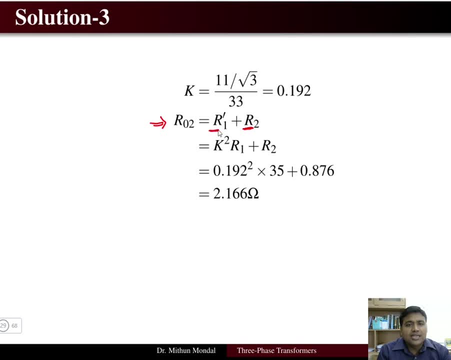 have to find the parameter R1, which is taken on the secondary side. So that is equal to k square R1, where k is the transformation ratio and R1 is given to be 35. Ohms and R2 is given to be 0.876 ohms. So on substituting, we get 2.166 ohms. Now on the star, 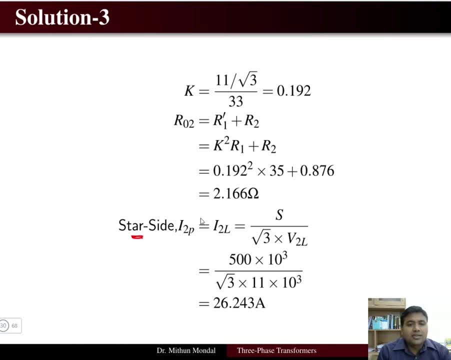 side, we know that the phase current and line current are one and the same. So we have the phase current and line current on the secondary side, which is the star connected machine is same, which comes to be the complex power S divided by root 3 times the voltage, and the voltage will be the. 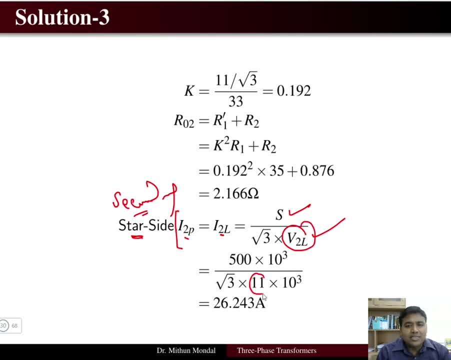 line voltage. So we have been given the phase current and line current on the secondary side, given 11 kV as the line voltage and power is 500 kVA power. So that gives you 26.243 ampere as the current on the secondary side, which is both phase and line, are equal to each other. Now, first we 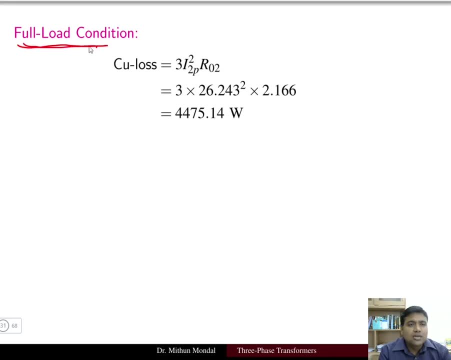 will take the full load condition and then we move to half load condition. So under the full load condition the proper loss is given by the formula 3 times I square R02.. So the net resistance that will be delivered to R02 is something like this. So this is not going to be the normal load condition. 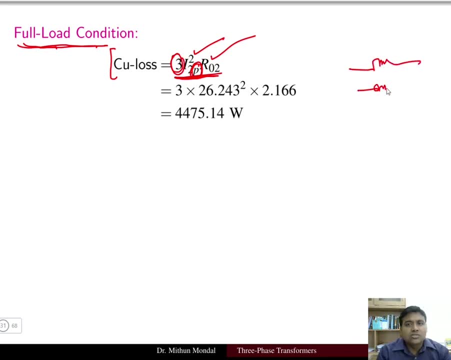 of the transformer which has been given here. We just need to find out the loss placed on the secondary side of the transformer and what is the current flowing on the secondary side. and this is the phase current we are dealing. So 3, we are multiplying because we have 3 conductors. So seeing, 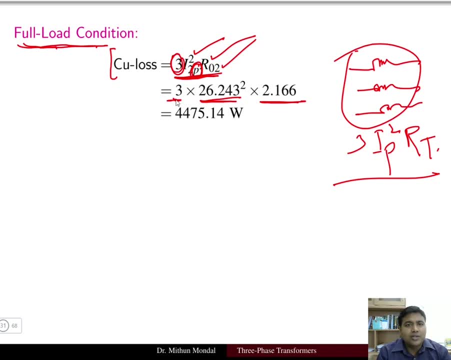 24 and three conductors are there. so three times we have multiplied. so that gives you 44- 75 watt. iron loss remains that same 3050 watt which is given in the question. so total loss is basically the sum of iron loss plus copper loss, which comes to be 75- 25 watt. now we have to find the efficiency. 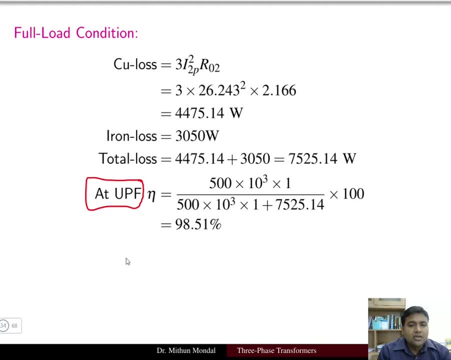 at two different condition. one is unity power function condition. so general formula of efficiency is x times the output power multiplied by the power factor, divided by the x into output, into power factor, plus the total losses. so total losses is the sum of iron loss plus copper loss. so here: 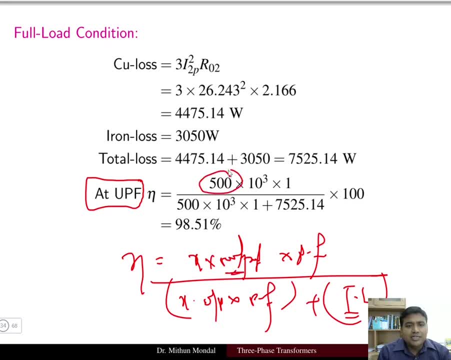 the output is basically 500 kva power factor under unity power factor condition is one and we are giving x equal to one for the full load conditions. so the iron loss and the copper loss together make up to be 7525 watt, which gives the efficiency to be 98.51 percent. however, at 0.8 power factor condition we have to substitute 0.8. 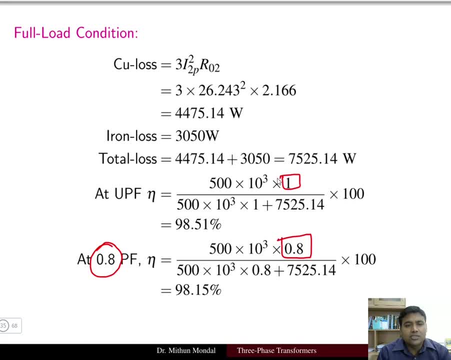 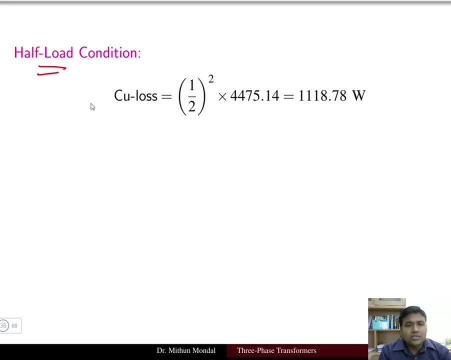 instead of one, which was the power factor unity, power factor condition. and here also we have to substitute in the denominator, which give you 98.15 percent. the losses remains the same because we are dealing with the full load condition. now for the half load condition. first, the copper loss will change. so copper loss will be half square multiplied with the. 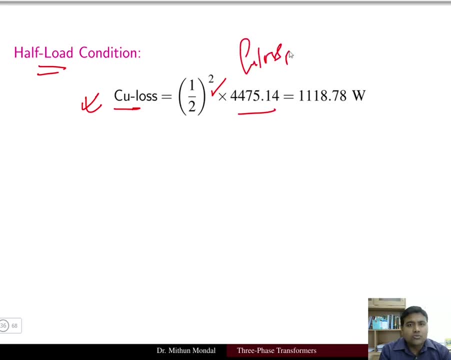 full load copper loss. so this is the copper loss which is under the full load condition, multiplied with half square, so it gives 1118 watt. then the total loss, which is the sum of the iron loss plus copper loss, iron loss will remains the same irrespective of the loading and 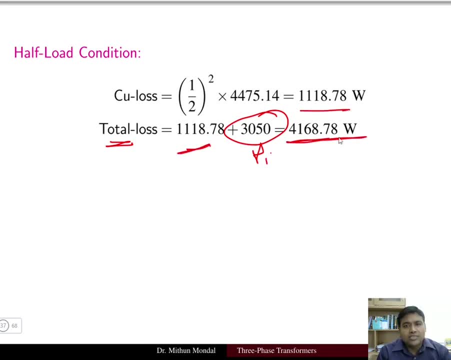 copper loss. we have calculated so total loss is 4168 watt. then at unity power factor condition we have to substitute what is the total loss on the machine and the power remains the same: 500. so one important point is that since it is half load, so the value of x we have to substitute as 0.5. 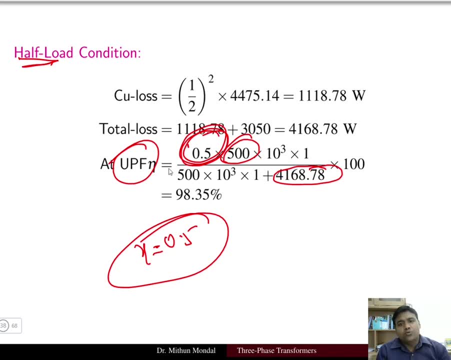 so here it will be 0.5 as the output power. so here also we have to substitute 0.5, multiplicate so it comes to be 98.35. okay, now, at the condition of 0.8 power factor. so only thing will change is 0.8. 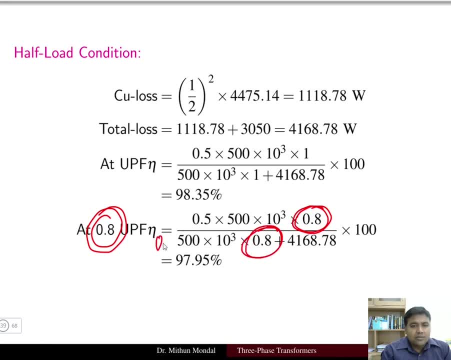 here the power factor and here you have the losses: 4168.78. that gives you to be 97.95 percent. so whether it is a full load or a half load, we can calculate the efficiency. under the full load, condition x will be 1, and under the half load we have to substitute the power factor. so this is: 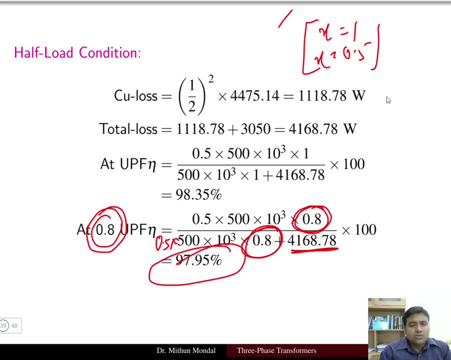 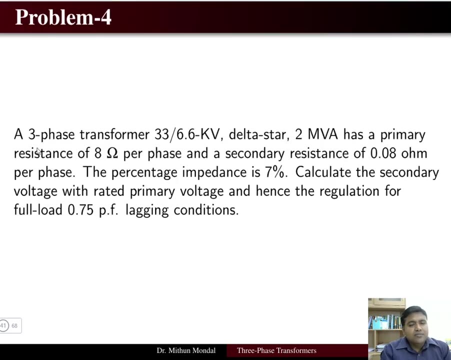 x will be 0.5, so copper loss is the one which is changing. so copper loss and different loading condition will be equal to x square times the full load copper loss, iron loss remains the same problem. fourth, you have a three-phase transformer, 33 by 6.6 kb delta star. so this is basically your. 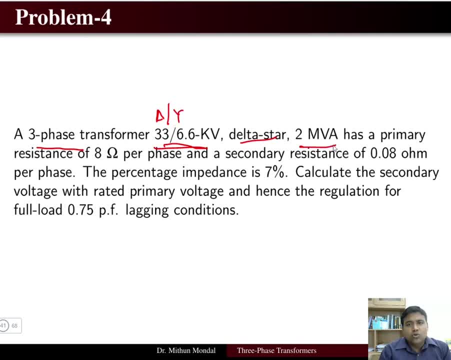 delta and this is your star 2 mva. so this is your complex power of the three-phase machine has a primary resistance of 8 ohms per phase. so you have r1 is equal to 8 ohm and secondary resistance r2 is equal to 0.08 ohms and this will be per phase, corresponding to per phase. 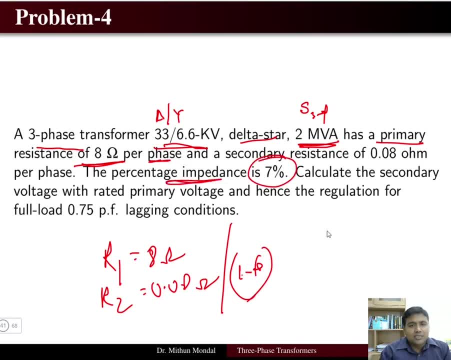 the percentage impedance is given to be 7 percent. so impedance percentage: if you calculate you can see that this is the resistance of the three-phase transformer: 33 by 6.6 kb. delta star given is 7 percent. calculate the secondary voltage with rated primary voltage, so v1 is 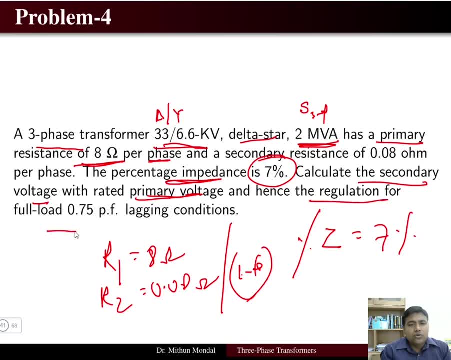 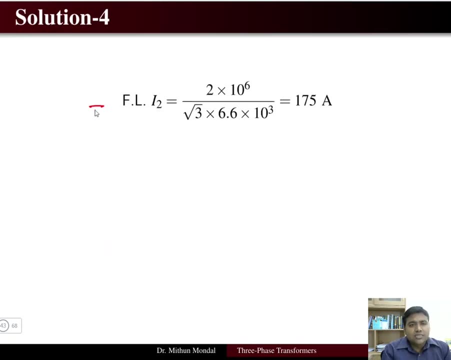 under the rated condition. hence the regulation for the full load. so under the full load condition, 0.75 power factor condition, what is the regulation of the machine and what is the rated primary voltage of the machine? so first we'll start for determining the full load secondary current of. 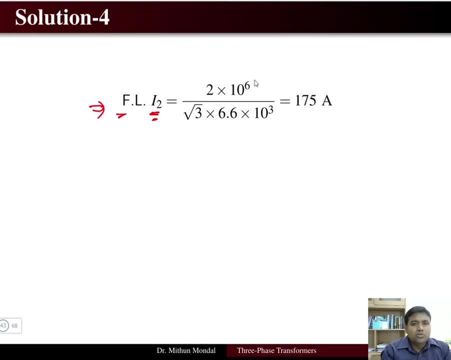 the transformer. so knowing the power formula. so the complex power s is 2 megawatt. so this is your s root. 3 by this will be your line voltage. so line voltage comes to be 6.6 kb. so that gives you 175 ampere as the line current. 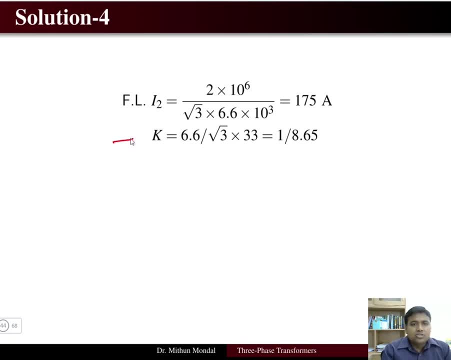 on the secondary side. so transformation ratio k will be in terms of the single phase. so convert the voltage on the primary side and the secondary side in phase voltage and then you obtain. so voltage will be 66.6, by root 3, and then you divide it be 33, so you get 1.865 as the transformation. 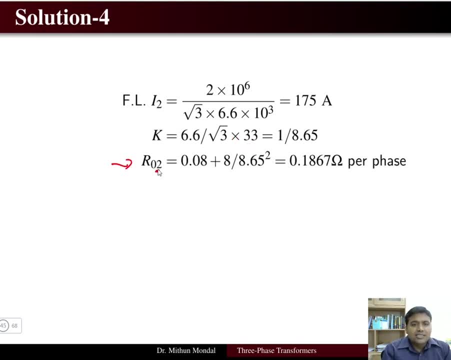 ratio. now the total resistance referred to the secondary side will be equal to r2 plus r1 dash. okay, so this r2 and r1 dash will be equal to k square times r1, because we are moving to the secondary side. so k square you can calculate from the transformation ratio. 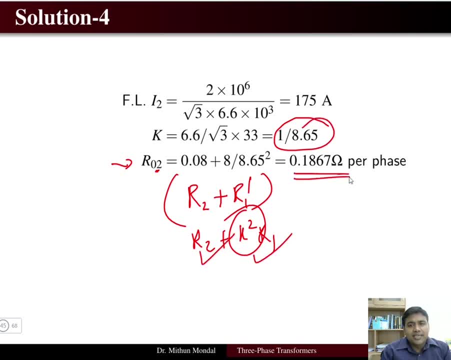 and R2 and R1 are given to you. So that gives 0.867 ohms and it is per phase calculation. So impedance drop is basically 7 percent, which was given for the total amount of the voltage, 6600, by root 3, that is the phase voltage. So total impedance drop is 266.7 volt. So 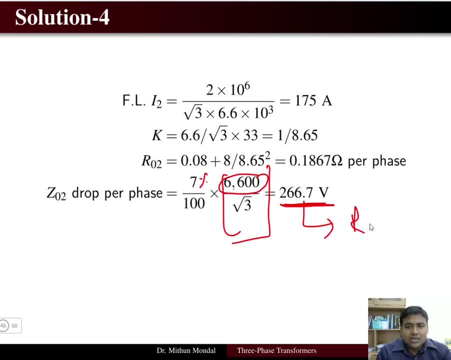 these drop is corresponding in the resistance plus the reactance. So this multiplied with the current, Now the impedance Z02 will be equal to the total voltage divided by the total current. So the voltage is basically 266.7, which is the voltage drop divided by the current on the 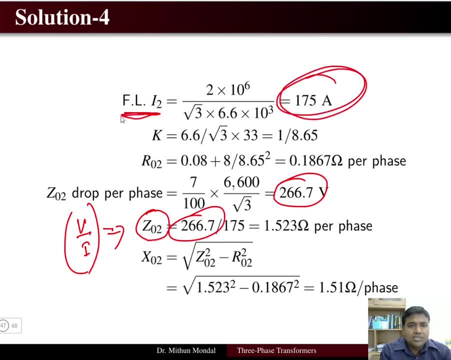 secondary side that we have calculated full load current on the secondary side that is 175 volt. So this gives 1.523 ohm per phase. Now we know that the Z is equal to R plus JX, So R is known. 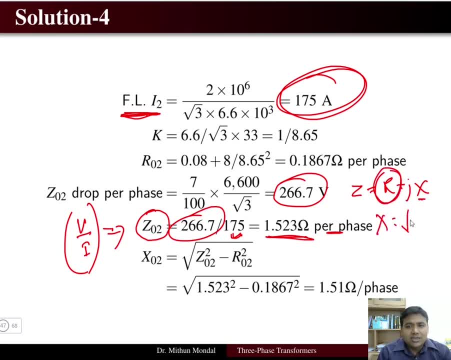 to us. X is not known to us. So X is basically under root of Z square minus R square. So Z02 square minus R02 square will give you the net reactance on the secondary side. So Z02, you have calculated. 1.523 square, R02 is calculated. 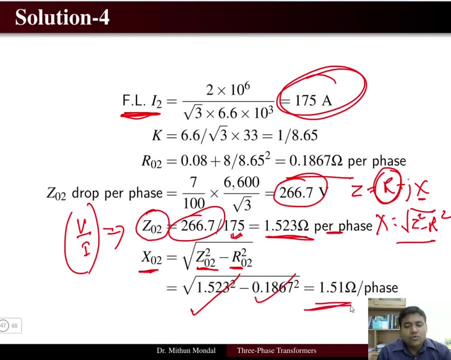 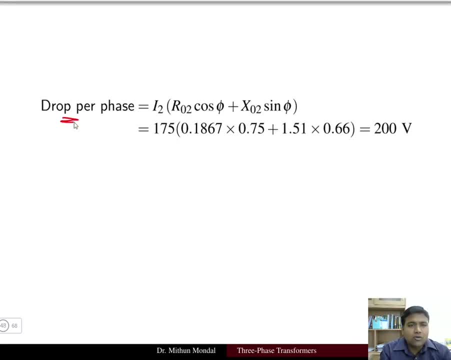 So R02 is calculated as 0.867 square, So it gives 1.51 ohm per phase as the total reactance of the machine on the secondary side. Then the drop per phase formula is basically: I2, R02 cos phi. 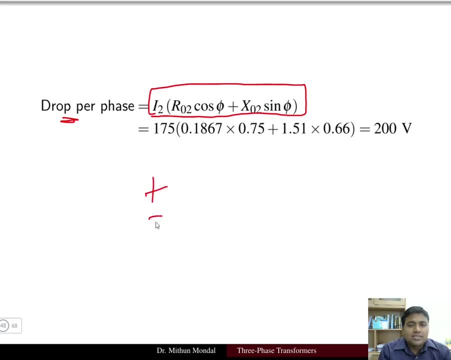 plus X02 sin phi. So plus minus sign comes plus for the lagging load and negative for the leading load. So here you have a plus sign because of lagging load condition. So you just substitute the value of the current I2, which is 0.867 square. So you just substitute the value of the current. 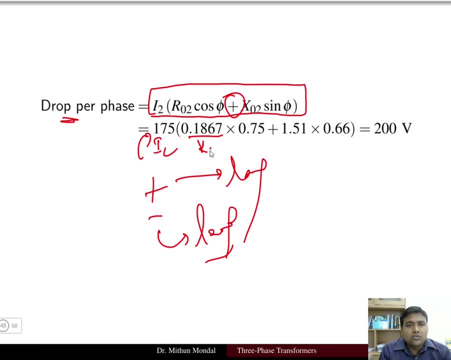 I2, which is 175.. R02 is equal to 0.1867.. Power factor cos phi condition is 0.75.. So correspondingly, this is for sin phi and X02. we have obtained, So we get the value is 200 volt as the drop. 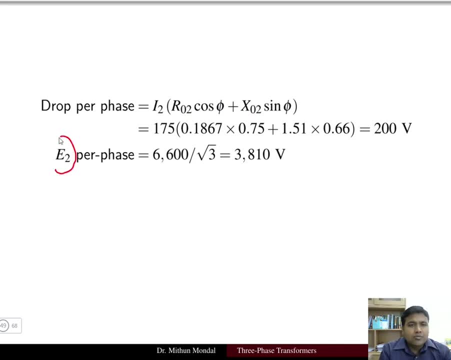 per phase. Then the induced EMF per phase is basically the voltage 6600 by root 3. that is the per phase we are calculating. This gives you 3810 volt because 6600 was the line voltage and it is a star connected. 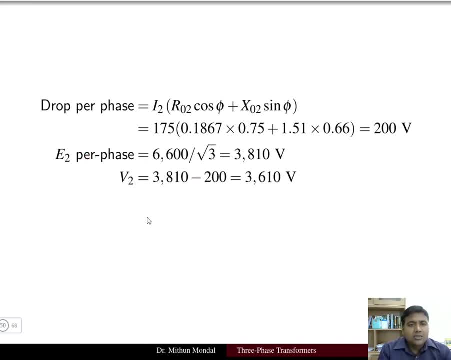 machine. So you have to divide it with root 3.. Then the V2, that is the voltage on the load side, is basically what is E2 minus the voltage drop. So E2 is basically 3810 and the drop is 200 volt. So you get 3610 as the voltage on the load side. So secondary voltage on 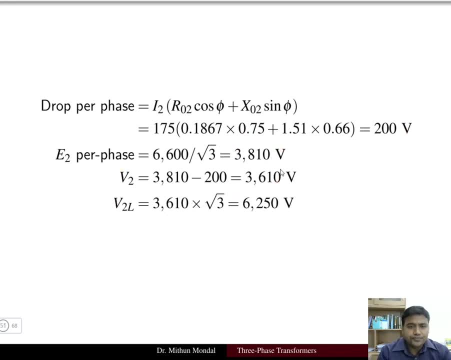 the load side is basically 3610 volt. Now this is your per phase voltage. You have to convert in terms of the line voltage, So multiplied with root 3, because line voltage will be root 3 times phase voltage for a star connected machine. So whatever the phase, 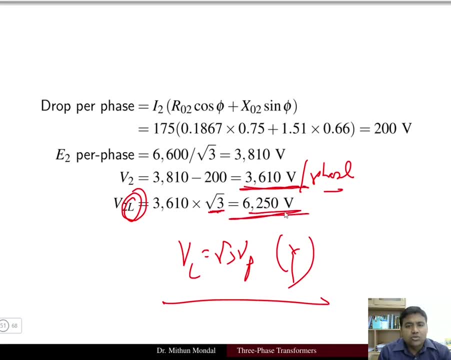 voltage we have got multiplied with root 3 will give you 6250. that is the voltage on the line side. So the regulation of the machine is basically 0.10.. What is the voltage drop? So voltage drop on the machine divided by the divided. 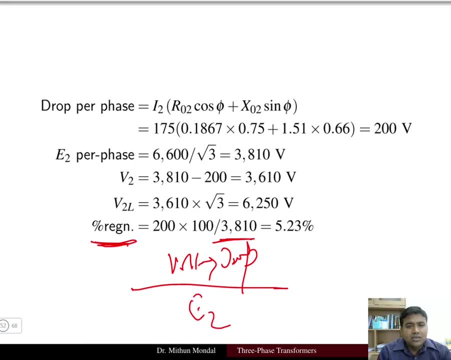 by the voltage E2 under the no load condition. So voltage drop: we have already calculated it is 200 and the E2 value that we have calculated per phase is basically 3810. multiplied with 100 will give you the percent, that is 5.23 percent as the regulation. 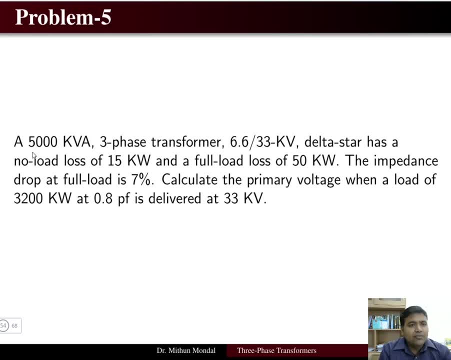 So problem fixed. You have a 5000 kVA three phase transformer, 6.6 by 33 kV, So delta star. So primary side is delta and secondary side is star. No load losses of 15 kilowatt. So 15 kilowatt is. 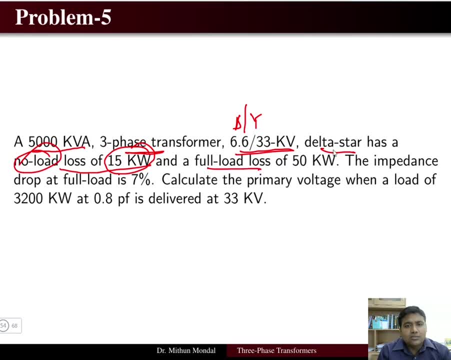 under the no load condition, the loss and full load loss is 50 kilowatt. So full load condition: the loss is 50 kilowatt. Impedance drop under the full load condition is 7 percent. Calculate the primary voltage. So you have to calculate V1 when a load of 15 kilowatt is under the 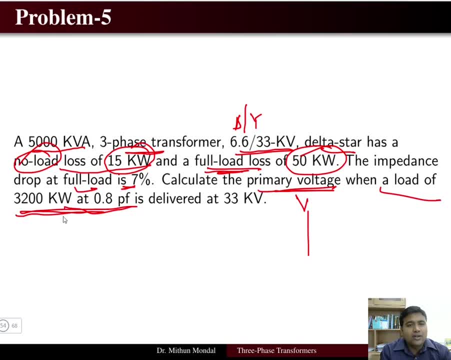 ñ of 32 kilowatt. 100 kilowatt at 0.8 power factor is delivered at 33 kV, So this is equal to V2 and this is the power of the load and the cos 5 condition. So first of all, 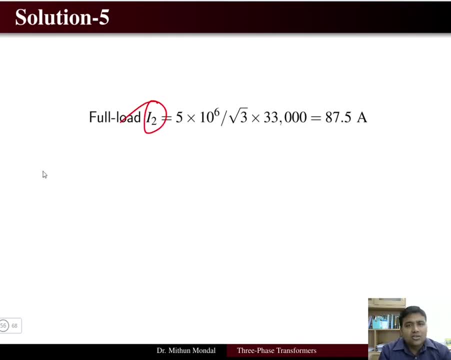 we will calculate the current which is flowing on the secondary of the transformer, So give with a given load conditions. So we have been given 5 kilowatt, So 5 into 10 to the power, 6 divided by root, 3 into 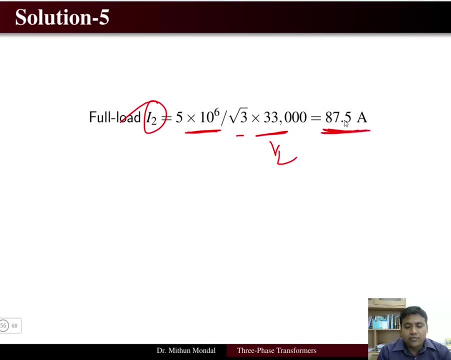 the voltage VL, So that is given as V2.. And since the current is flowing with the current of the transformer, give you it is 67.5 ampere. impedance drop per phase is 7 percent of the net voltage which is per phase. so per phase you have 33 kV as the line voltage divided by root 3, so 7 percent of 19 kV. 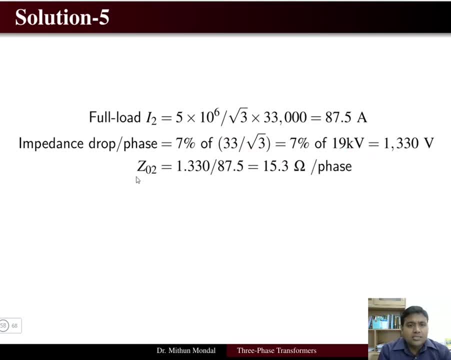 which keeps to be 1330 volt and Z02 will be then the voltage divided by the current. so voltage is 1330 volt divided by the current, then you get 15.3 ohms per phase as the impedance. full load copper loss is basically the total losses minus the losses that is being taken in the 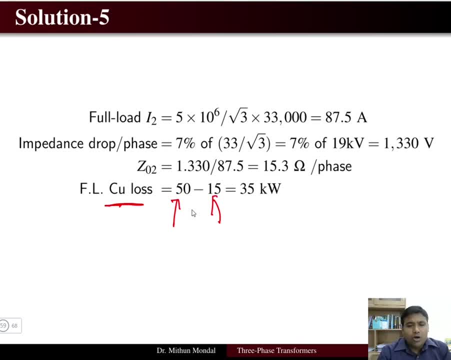 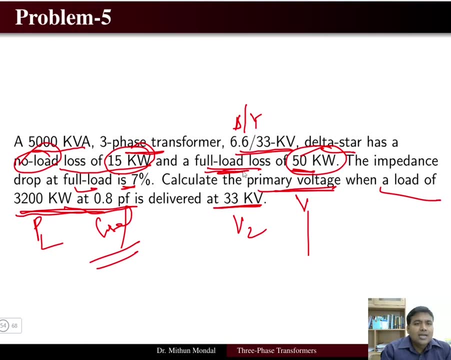 no load condition. so that will be the copper loss at full load condition. because here in the problem it has been given that full load loss is 50 kilowatt and no load loss is given to be 15 kilowatt. so the subtraction is 15 kilowatt, so the subtraction is 15 kilowatt, so the subtraction 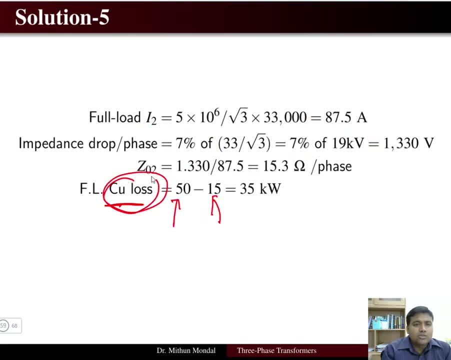 of that will give you the full load copper loss. so 50 kilowatt is the total loss minus the no load losses, so no load condition. it will be, you know, the iron loss basically. so that gives to be 35 kilowatt. so this 35 kilowatt if we substitute as 35,000, so this is basically the full load. 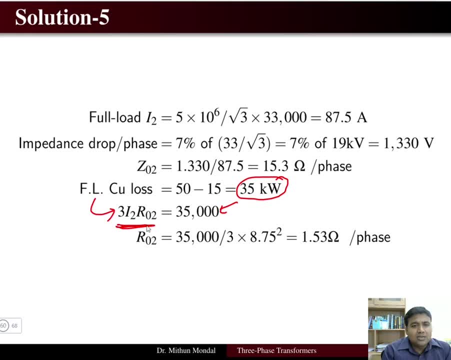 copper loss. so we have three conductors and the current flowing is I2. so here square will be there and the current flowing is I2, so here square will be there and the current flowing is I2. so here and R02. so R02 is the total resistance on the secondary side, so we can easily obtain what is. 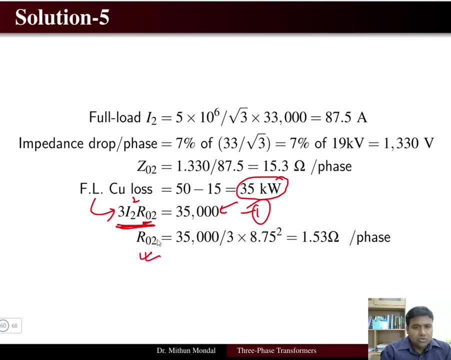 the value of R02 from this equation, because we know what is the value of the current, so we get 1.53 ohms per phase as the total resistance and the total reactance impedance also. we know it, so it will be easy to find what is the total reactance of the machine. 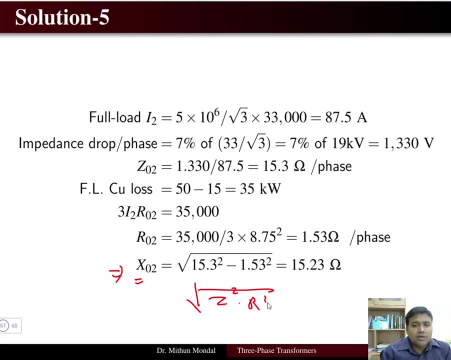 or with a under root z square minus of r square, so z being the 15.3 ohms per phase and the resistance is basically 1.53 ohm. so z minus z square minus r square will give you under root 15.23 as the net reactance of the machine, then the load. 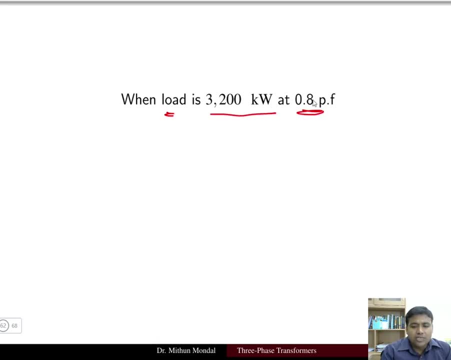 information is given to be a 3200 kilowatt and 0.8 power factor. you can calculate what is the current flowing through the load. so this is your load. here you have the current I2, so this current is, basically you can easily calculate power is equal to root 3 VL IL of. 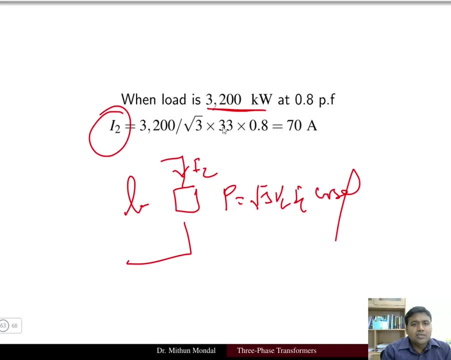 cos phi. so here the power is 3200 kilowatt. so you can substitute 3200 into 10 to the power 3 and you have root 3 multiplied by the voltage. so voltage you have seen that is 33 kV on the. 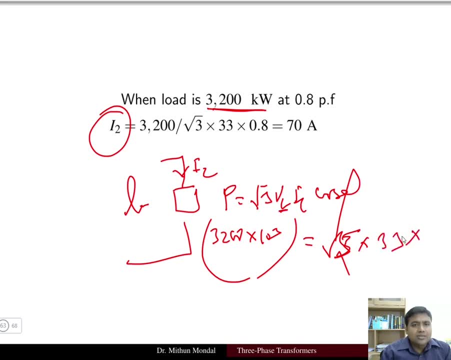 start side. so 33 multiplied with the current- that is what we have there that you need to calculate into cos phi is 0.8, so we can easily get what is the value of the current. this is the line current that is flowing. so it is 70 ampere now the drop that you can calculate, since it is a start side. 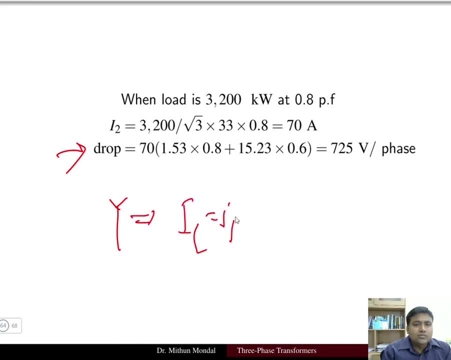 machine, your line voltage will be equal to phase current. line current and phase current are same, so 70 ampere will be remaining the same. now plus sign is coming here for the lagging condition of the load, which is having a power factor 0.8 and cos phi and sine phi. 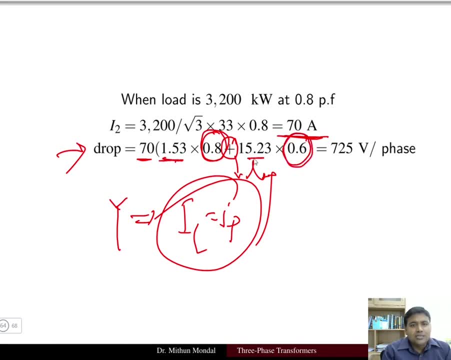 is 0.6. this is the resistive drop and this is the reactive drop. so 725 volt per phase is the total drop on the machine. then the regulation you can calculate as the drop, 725 volt divided by the net voltage of E2 under the no load condition into 100, will give you 3.8 percent. 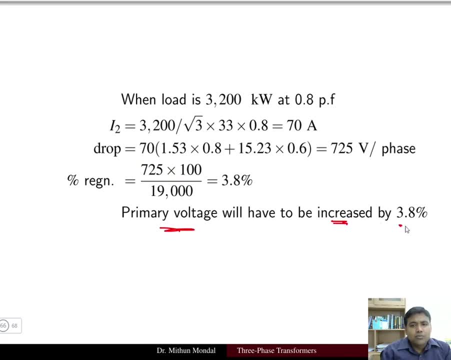 now primary voltage will have to increase by 3.8 percent because the regulation is 3.8 percent, so primary voltage will have increase of 3.8 percent. so whatever 3.8 percent of the primary voltage, whatever you have multiplied plus the primary voltage, V1, so V1 plus 3.8 percent. 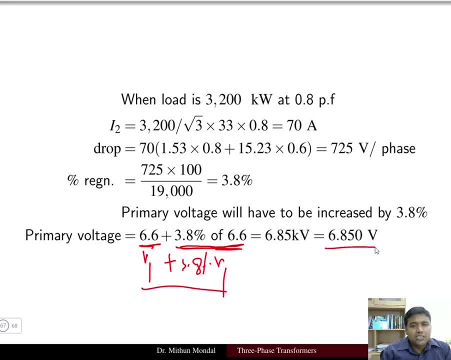 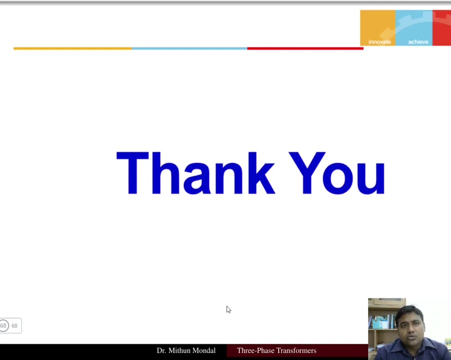 of V1 will give you the net primary voltage of the transformer. so this gives you 6.850. so this is your E1. we can take E1, so we will get 6.850.. volt. That's complete the tutorial on three-phase transformer. So here we have taken all the concept.